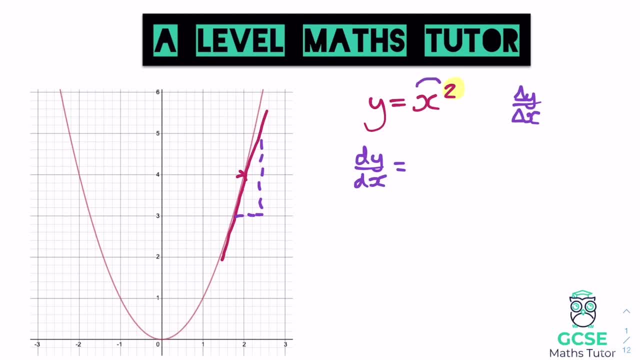 that by the coefficient of x, that's before it Now, the coefficient of x squared is one at the moment. so one times two gives us two. okay, and then we reduce this power here by one, so it's two, and that just goes down to the power of one. so it's 2x to the power of one, and obviously. 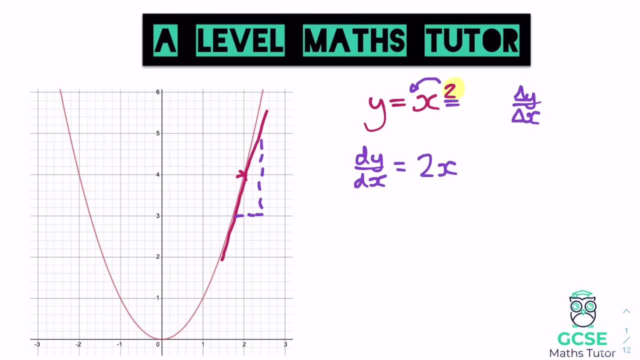 when we have a power of one, we don't need to write it. So there we go For a nice, simple graph like x squared. that would be our expression, that is our value of dy over dx, there 2x, and we can. 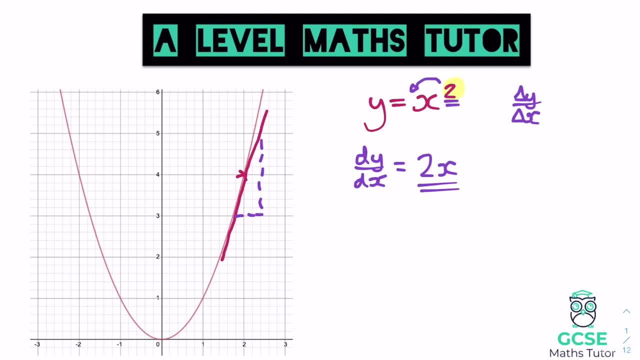 use that to find out the gradient at that point on a curve, and we're going to look at all of these steps as we move along, but here's a bit of an overview on a nice simple one. If I wanted to find the gradient at that point there that we've already highlighted, that has an x coordinate of 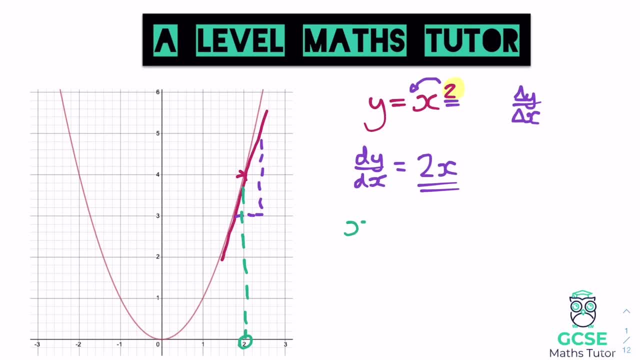 two. okay, so we take two and we'd sub it in. and when x equals two, 2x or dy over dx equals two, lots of two or two times two, which is four. so the gradient at that point would equal four. 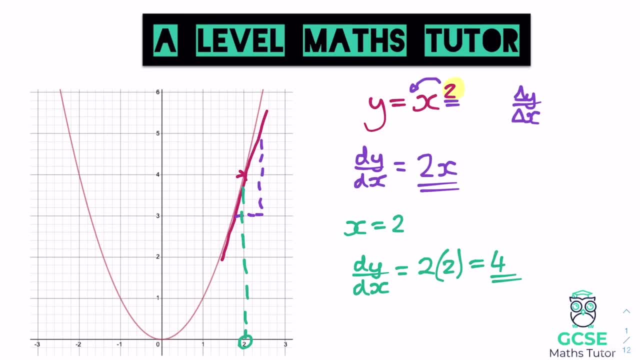 Now, these are all the things that we're going to have a look at. throughout this video, We're going to have a look at obviously differentiating, much harder graph equations than this one, and then we're going to have a look at subbing some values in to work out the value at those particular. 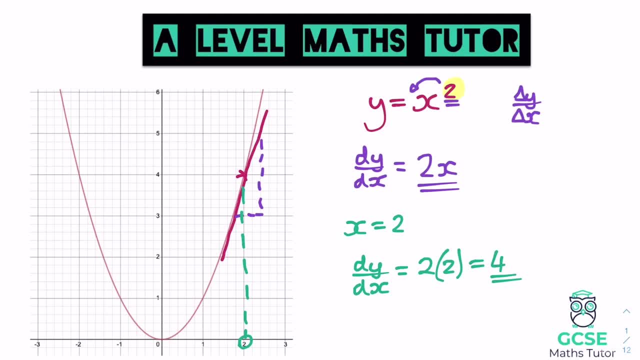 points. okay, But that's a bit of an overview of what we're going to look at in the next video And the process that we're going to go through. obviously, if you've never seen differentiation before, but it's quite nice and simple: Multiply the coefficient by the power and reduce the power. 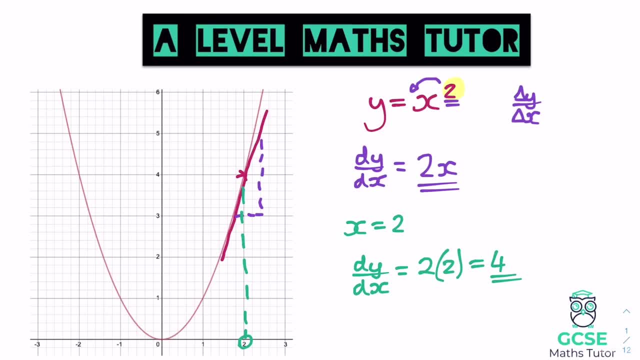 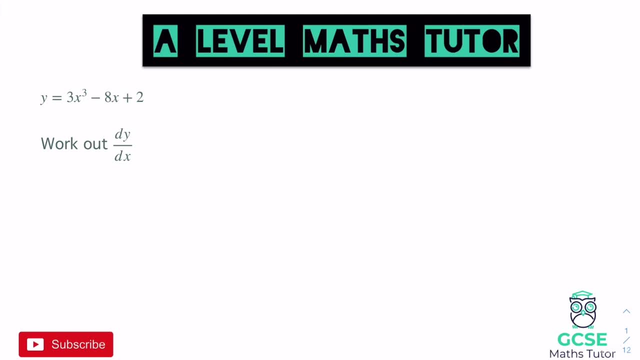 by one. That is pretty much all we're going to need to do, So let's have a look at a couple of different questions where we're going to be following this process. Okay, so for our first one here we have: y equals 3x cubed minus 8x plus 2, and it says: work out dy over dx. So let's have 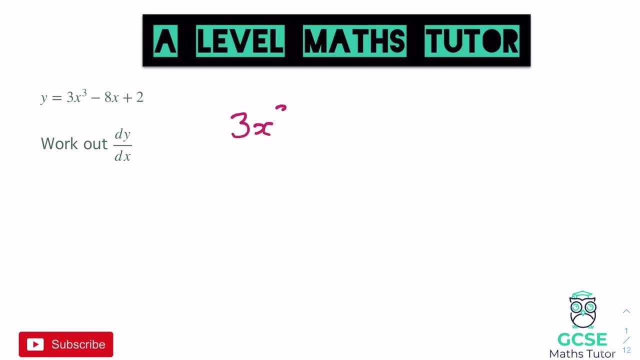 a look at what we've got. I'm going to write this out a little bit clearer: We've got 3x cubed minus 2.. Now let's go about actually following this process then. So for this one, our first power is 3 and our 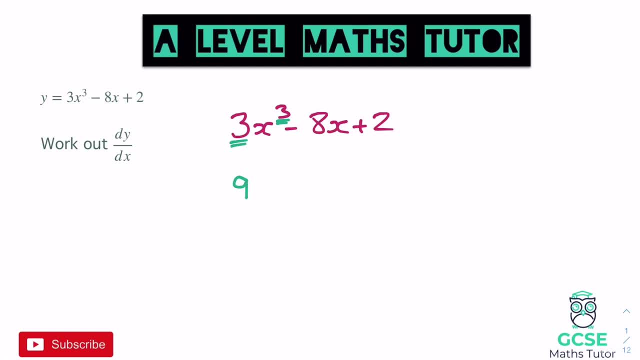 coefficient is 3.. So if we multiply those together, that gives us 9.. So we've got 9x. and if we reduce that power by 1, that becomes x squared. So we have 9x squared for our first piece. On to the next one. 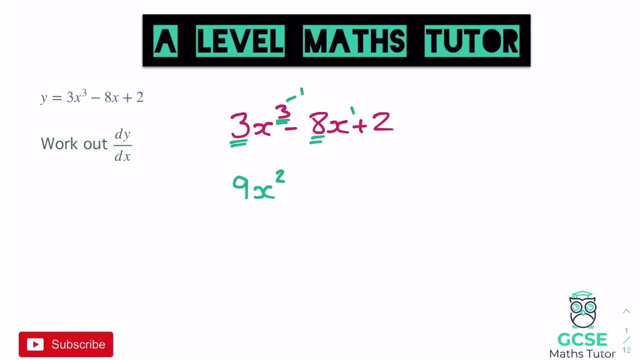 we've got a coefficient of 8 and, technically, a power of 1 there, because we obviously don't write that in when we have a power of 1.. So if we multiply those together we still have 8.. And if we reduce our power by 1, that goes down to 0.. x to the power of 0 equals 1.. Let's just write that. 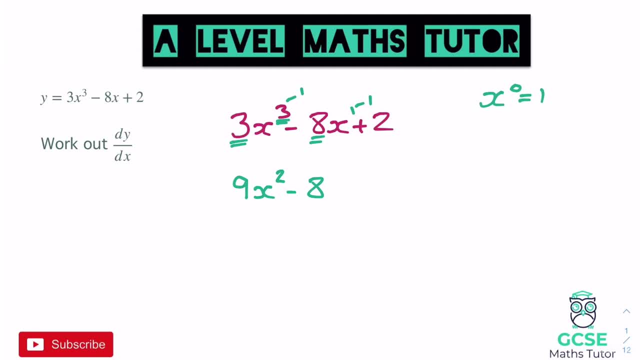 down x to the power of 0 equals 1.. So we don't actually need to put any x's with this 8 here, obviously, because that's just 8 times 1, which is 8.. On to our next one. Technically, there's: 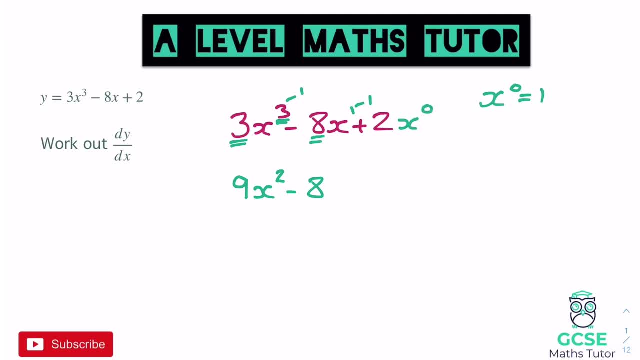 obviously no x there. We could actually write it as x to the power of 0., And 0 times 2 is 0, and the whole thing just disappears and becomes 0.. So when you've just got a number on its own, 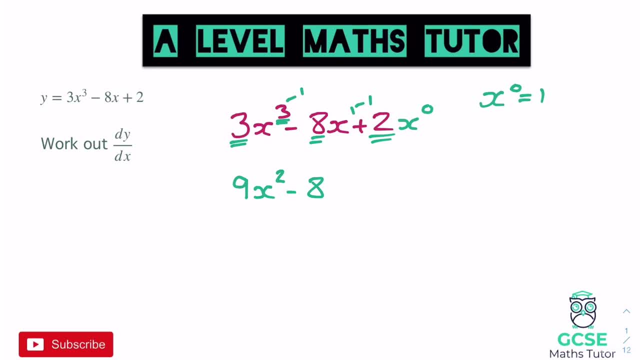 that's just going to disappear, okay. So obviously, only when we've got a number on its own. we have an x, a coefficient of x. there it's actually going to get multiplied, But obviously because the power of 0 is technically 0, sorry, the power of x is technically 0,. 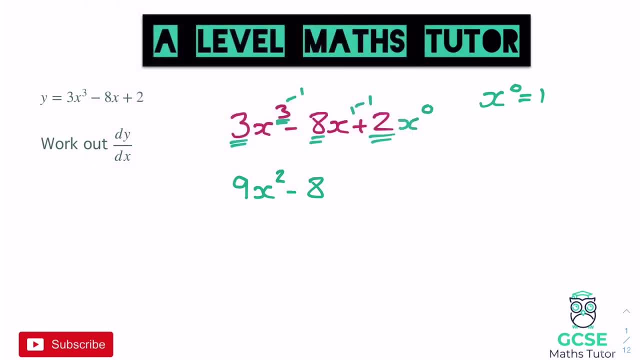 that just becomes 0.. And we end up with our final expression here And we would say: dy over. dx is equal to 9x squared minus 8.. And there is our final answer. So there we go. That's how we're. 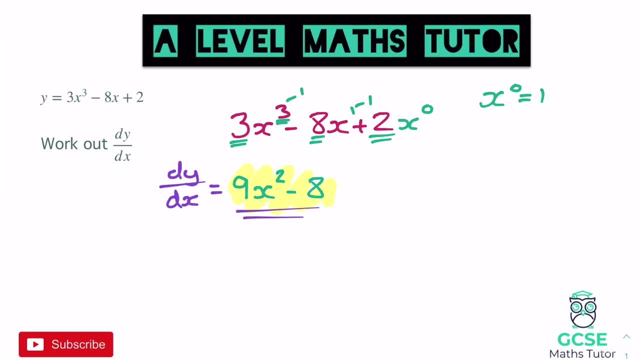 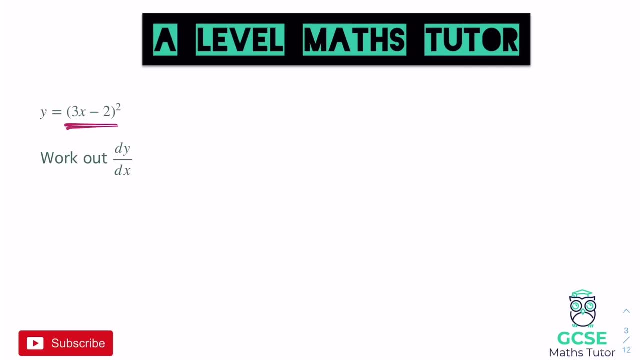 going to differentiate some of these expressions, Let's have a look at another one. Okay, here we go, So not necessarily any more difficult, but obviously we've been given this equation here, obviously already factorised in brackets. So before I differentiate that, 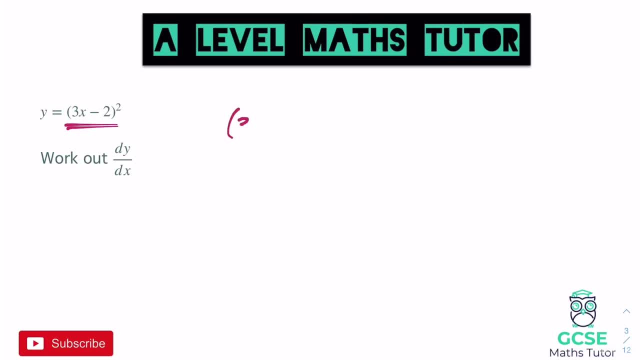 I'm just going to expand that out And obviously, remembering that, obviously all our little different bracket rules and double brackets and all those sorts of little different things that we've learnt at GCSE level, we're going to expand this one out. So I was actually going to rewrite. 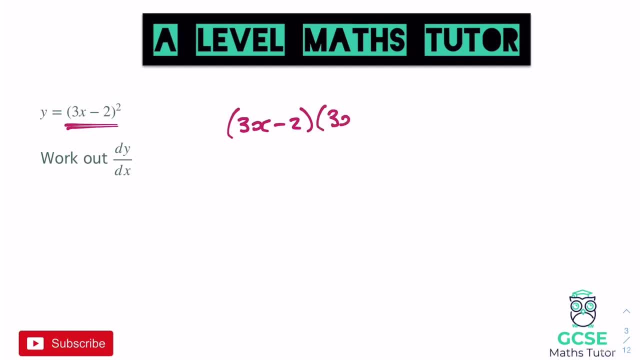 that as two brackets there. So let's rewrite this as a double bracket: 3x minus 2, 3x minus 2.. And let's expand that. So 3x times 3x is 9x squared. Then you have the two multiplications 3x times. 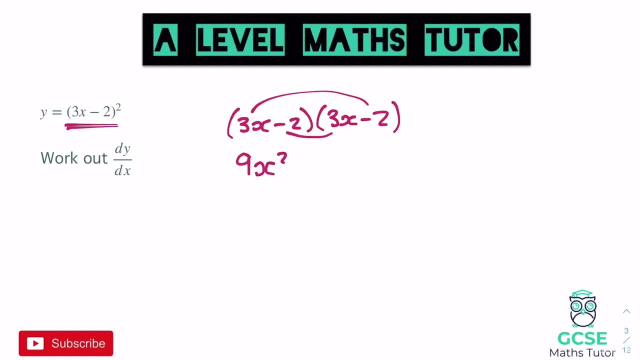 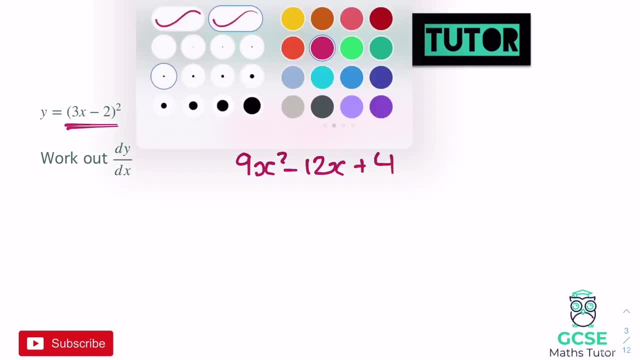 2 and minus 2 times 3x, both of those making negative 6x. So in total that's negative 12x. And then negative 2 times negative, 2 is positive 4.. And now we can go about differentiating it. So 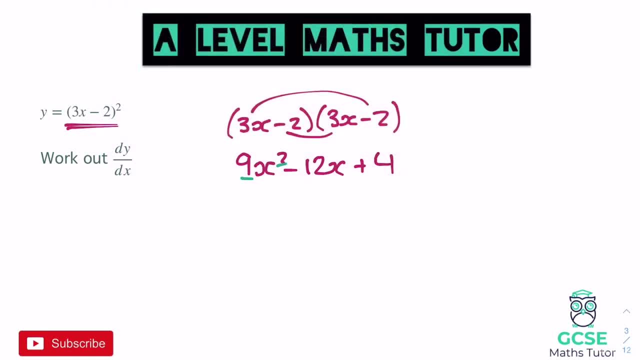 let's have a look. Our power here is 2 and our coefficient is 9.. So times them together, that becomes 18.. So 18x when we reduce the power by 1.. And then for the next one, obviously this: 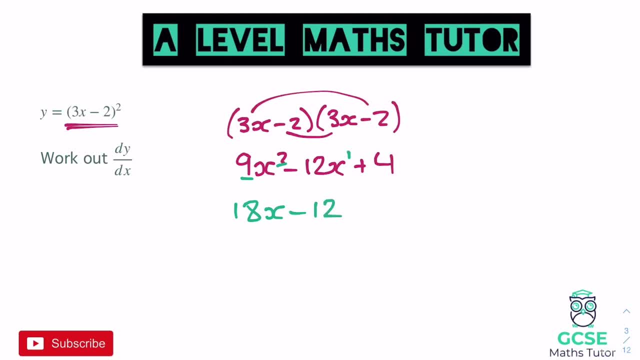 is a power of 1.. So that becomes minus 12.. And reducing the power by 1 gives us x to the power of 0.. And then for the last piece that just disappeared. So we're going to do that again. 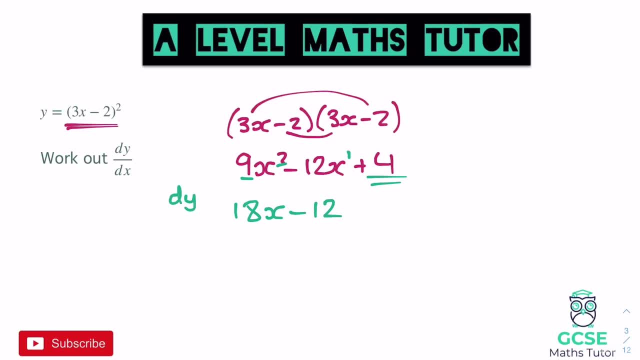 So there we go. There is our final expression. there We get dy over. dx is equal to 18x minus 2.. There we go Now. obviously, one thing I haven't mentioned is obviously why and how this happens, And I will link in the description below proof of why we differentiate the way we do and how. 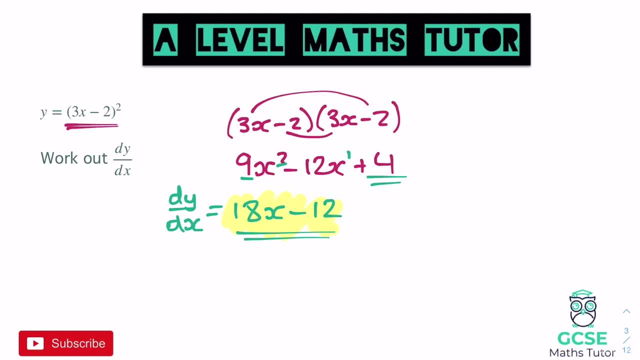 it's actually derived. So obviously do check that video out if you do want to see how and why this works, But otherwise we're just looking at this sort of practice type questions on exactly how you go about answering them. So before we go any further, I've got a couple of questions for you. 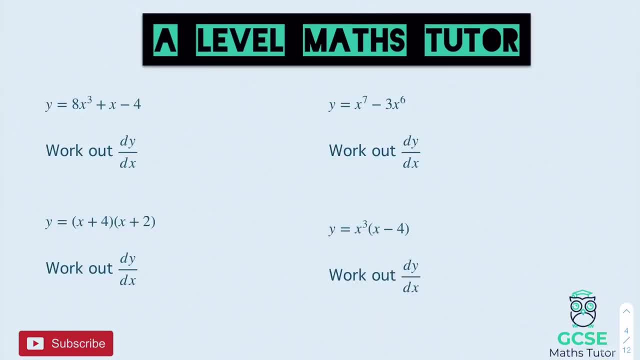 to have a go at. And here they are. Okay, so there's four questions there. So pause the video, have a go at all of these. I'll go over the answer in a sec. Okay, so for this first one, then Now. 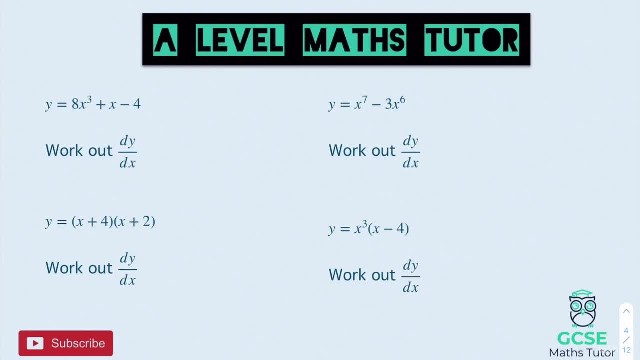 8x cubed. So if we multiply the coefficient by the power of 3,, 8,, 16,, 24, we get 24.. There we go, And that's 24x. Reduce the power, That becomes x squared For the next one, the power of x there. 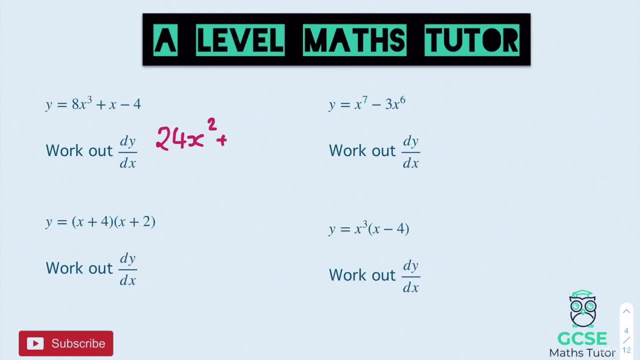 is 1 and the coefficient is 1.. So that's just going to become plus 1.. So that's just going to become plus 1.. And the power of x is obviously 1 at the moment. Reducing that to 0, that's going to be no. 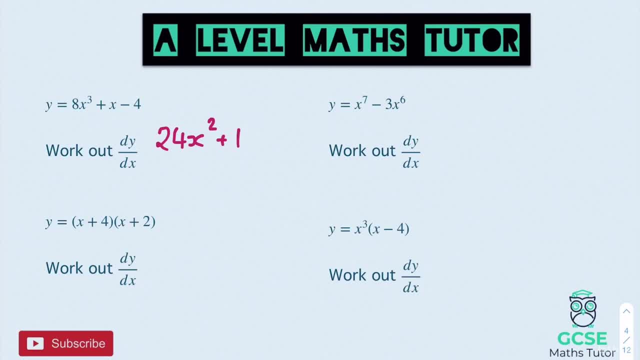 x's with that, And then the 4 at the end is just going to cancel out. Okay, so there we go. There is our first one done, 24x squared plus 1. Onto the right there, x to the power of 7. So multiply. 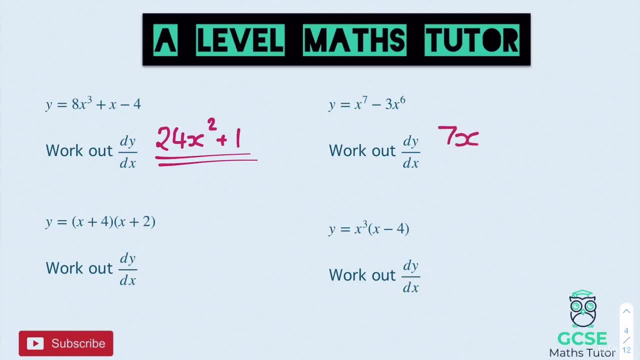 the coefficient, which is 1. We get 7x And reduce the power to a 6.. Onto the next part. we've got minus 3 times, the 6 becomes 18. And the power of x drops down to a 5.. There we go. So there's our 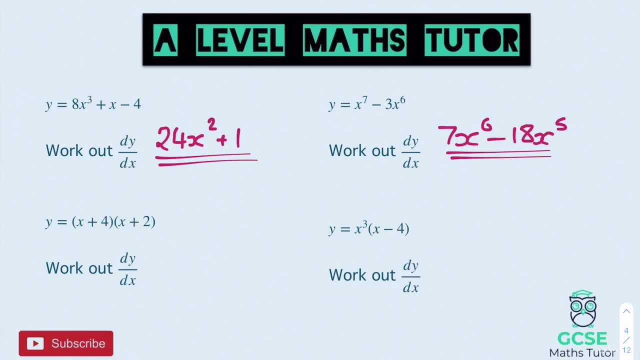 next one On the bottom left here we've got to expand this out first. So if we expand that out, we get x squared plus 2x plus 4x, which is plus 6x, And then 4 times 2 is 8.. And there we go. So 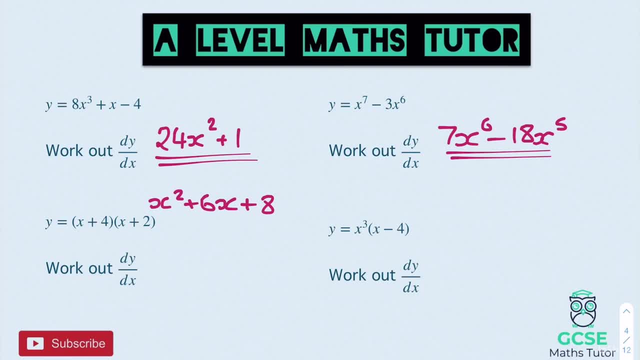 that's what we get when we expand it out. And now, if we differentiate it 2 times, the 1 gives us 2x, 1 times the 6 gives us 6.. And the x there disappears And our final piece cancels out. So 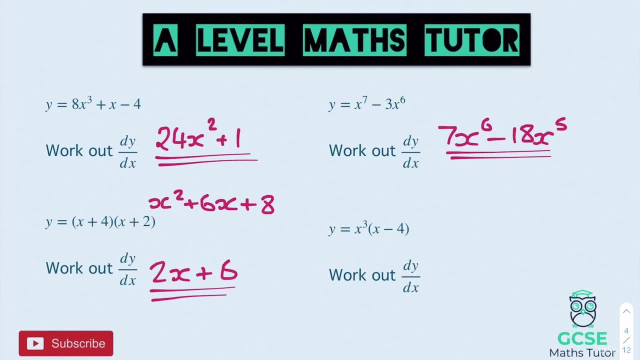 we get 2x plus 6.. There we go, There's our next one, And then for our final one here, we've got to expand the bracket out first, So x cubed times 6. And then we get 2x plus 6.. And then we get. 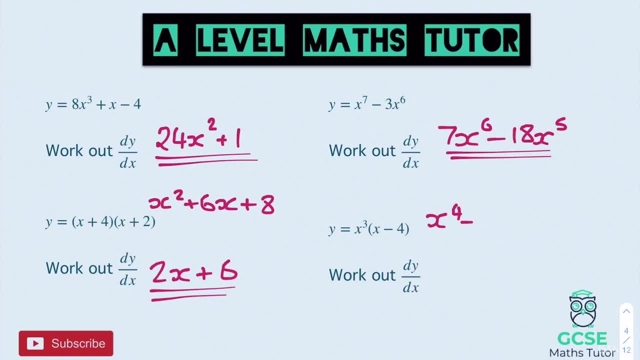 2 times x becomes x to the power of 4.. And then take away 4 lots of x cubed, And there we go, Just expanding that out, And now we can differentiate. So 4 times the 1 gives us 4x. 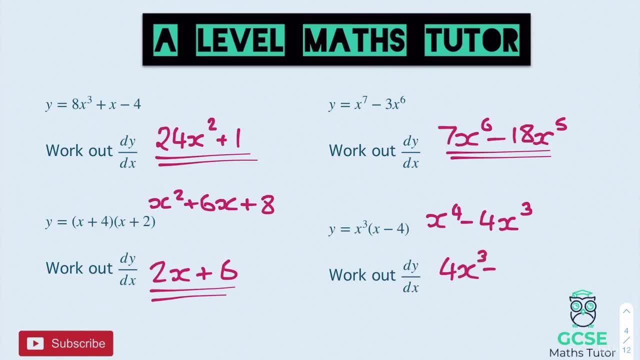 Reduce the power down to a 3.. And then, for the next bit, 3 times 4 is 12.. And reduce the power down to a 2.. All right, There we go. And that is that differentiated as well. OK, So there we are. 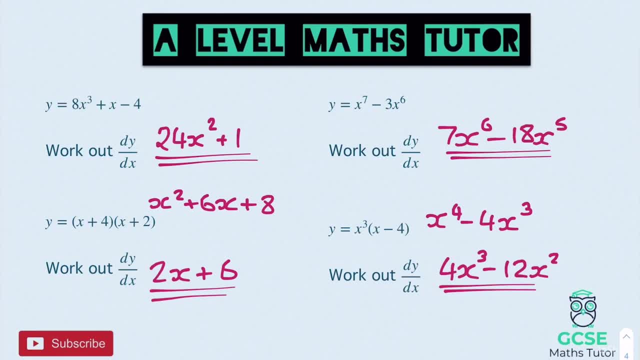 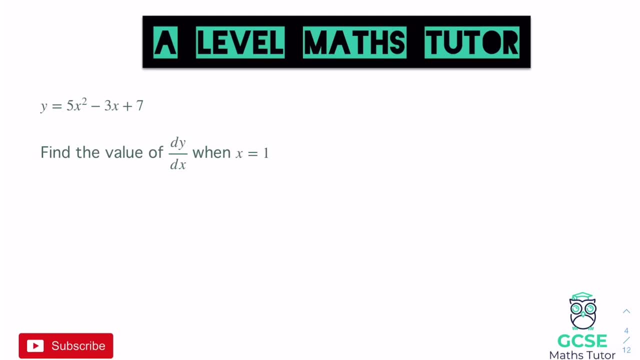 That's a little introduction onto some of the differentiating. Now let's have a look at some of the other aspects of this where we look at actually plugging in a value. OK, So for this part of the process, look, we've got. y equals 5x squared minus 3x plus 7. Find the. 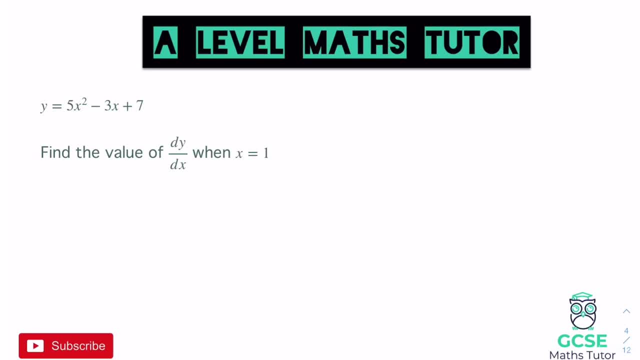 value of dy over dx when x equals 1.. Well, that's OK, Because all we have to do is differentiate and then substitute this value of 1 in. Now it doesn't ask it in this question, But that is what we're doing. We are finding the gradient of the tangent at that point where x equals 1.. But 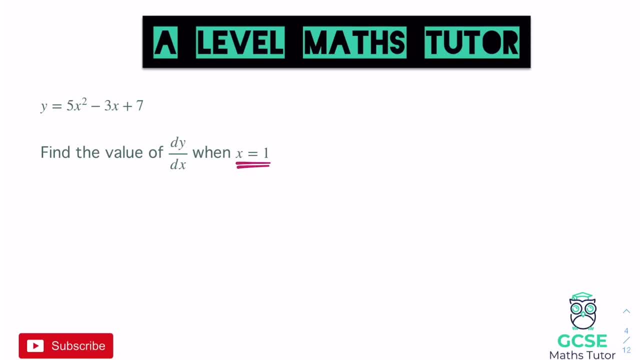 obviously we're not going to have a look at the graphical element or aspects of it just yet. We're just going to focus on part of the process and obviously some of these just mathematical processes at the moment. So for this part of the process, look, we've got y equals 5x squared minus. 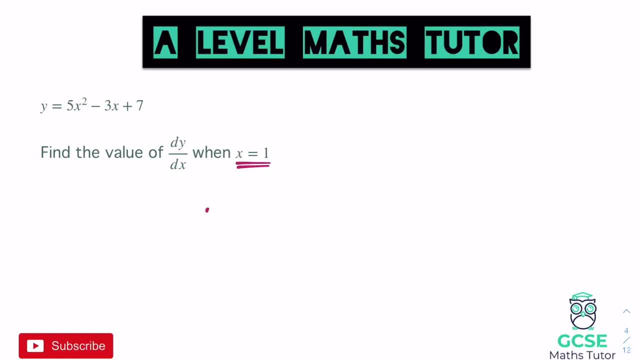 7.. So for that first one up there, times the 5 by 2 gives us 10.. So we get 10x And the power gets reduced to 1.. And then for the next bit, we have minus 3. And that power of x there is going to. 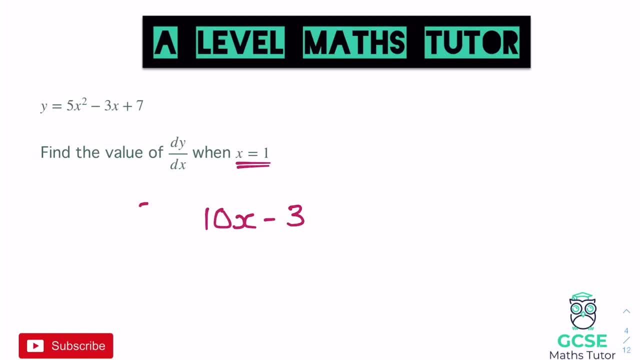 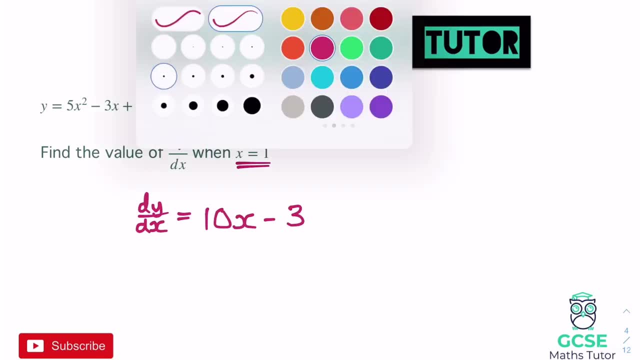 disappear. So we have 10x minus 3.. And let's just label that. So dy over dx equals 10x minus 3.. So when x is 1, all we need to do is substitute 1 in. So when x equals 1, we are going to get. 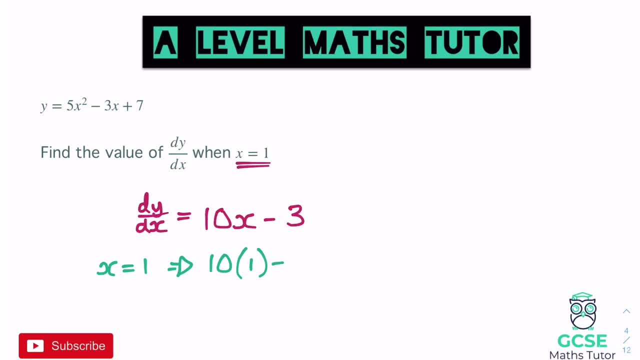 10 times 1.. Minus 3.. Okay, which equals 10 minus 3, which equals 7.. There we go. So that is our value there, when x equals 1.. There we go. So quite nice and simple. hopefully We're going to have a look at. 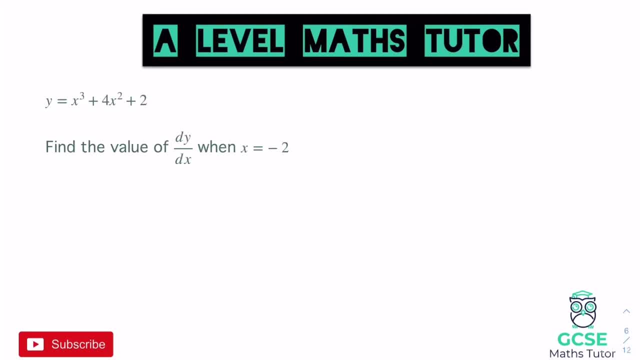 one more quick one before you have a go. So, following the same process, let's have a look at this one. So we've got x cubed up there. Obviously we're looking at this up just up here. So times the coefficient by 3, that gives us 3x, And reduce the power by 1 gives us a power of 2.. 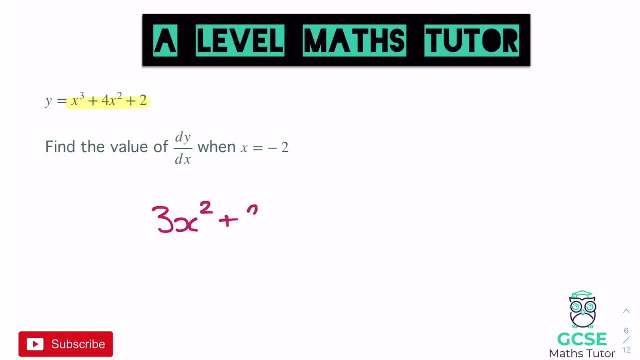 On to the next bit Times: the coefficient of 4 by 2, gives us 8.. And reduce the power by 1, gives us x, And then the 2 at the end is going to disappear, So that there is my dy over dx. Okay. So this obviously says: find the value when x. 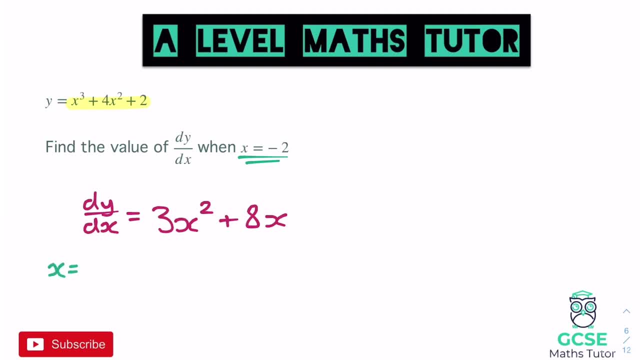 equals minus 2.. So when x equals minus 2, let's see what we get, There we go. So let's sub this in: We get 3 lots of minus 2, squared plus 8, lots of minus 2.. Now, obviously you can just stick this: 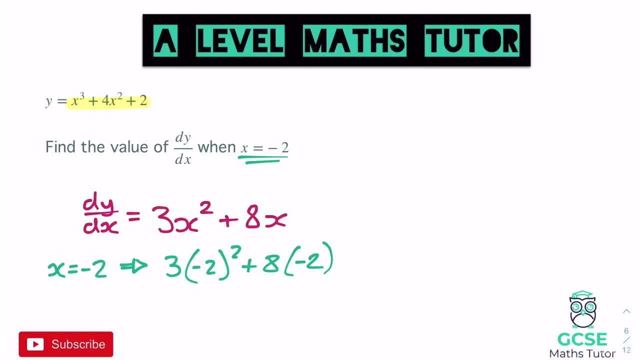 into the calculator, but I'm just going to go ahead and work it out. Minus 2 squared is 4.. So 3 times 4 is 12.. And then we're going to add 8. lots of minus 2. 8 lots. 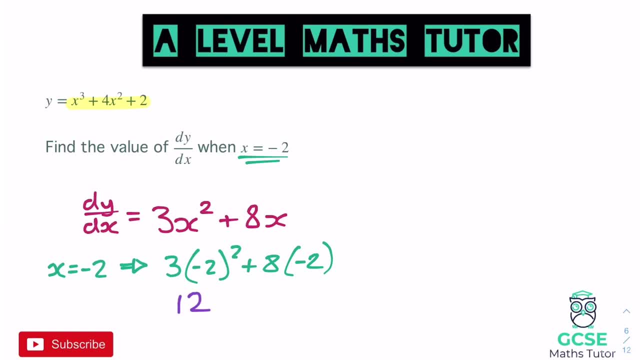 of minus 2 is minus 16.. So that is going to be add minus 16,, which is just minus 16.. 12 take away 16 is minus 4.. And there is our final answer. There we go. Obviously, you can stick that all. 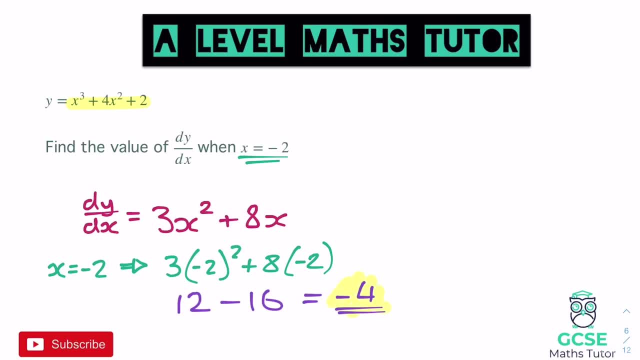 into a calculator, but it's quite nice and simple some of these, just to do them, obviously, rather than typing them in. Right, there we go. So that is what we're going to have a quick practice on before we have a look at some slightly harder questions to 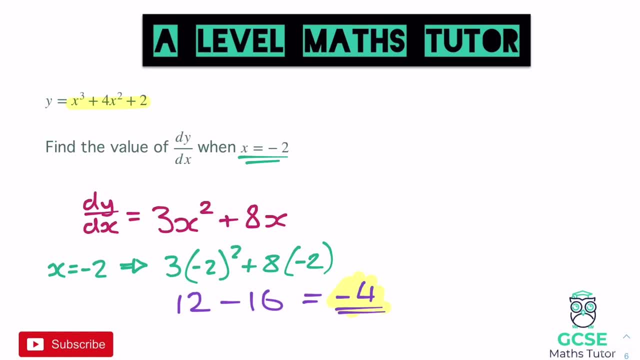 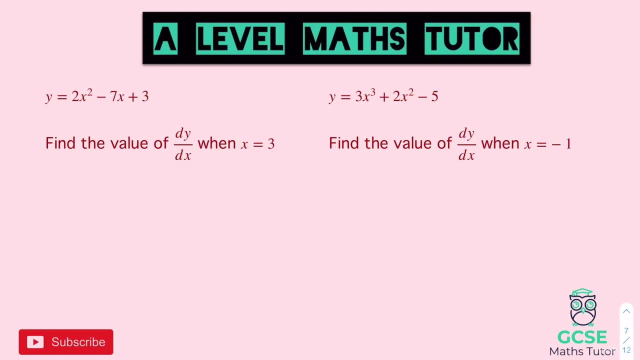 differentiate. So there's a couple here for you to have a go at before we move on. Okay, so here's two questions, So pause the video there, have a go, and we'll go over the answer in a sec. Okay, so for this first one then. So let's go about differentiating it. So when we differentiate, 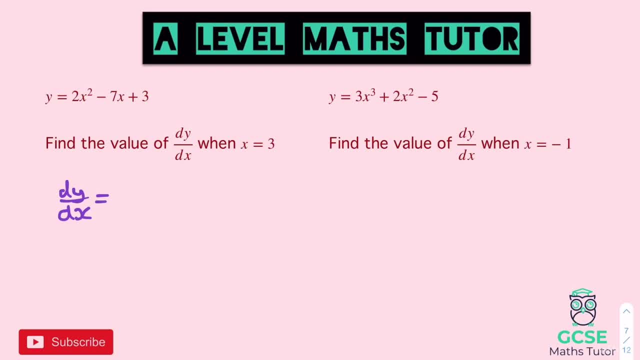 this one dy over dx is going to equal 2 times the 2 there gives us 4x, and the power gets reduced to 1.. And then 1 times 7 gives us 7, and that power reduces to 0. So that's going to disappear. 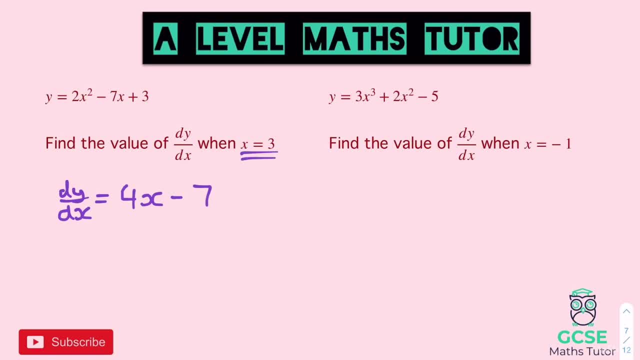 for that first bit. And then x equals 3 now. So if we sub x equals 3 in, we get 4, lots of 3, take away 7, which is 12, minus 7, which is 5.. And there we go. so there's our final answer: 5.. 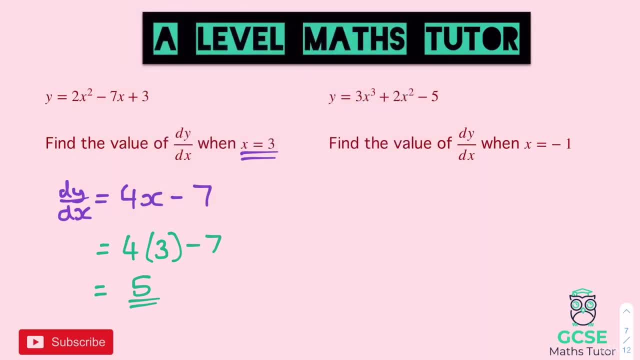 On to the next one. Let's have a look. So for this one here, if we do dy over dx, let's have a look. what we get. 3 times 3 is 9, reduce the power by 1, gets us x squared 2 times. 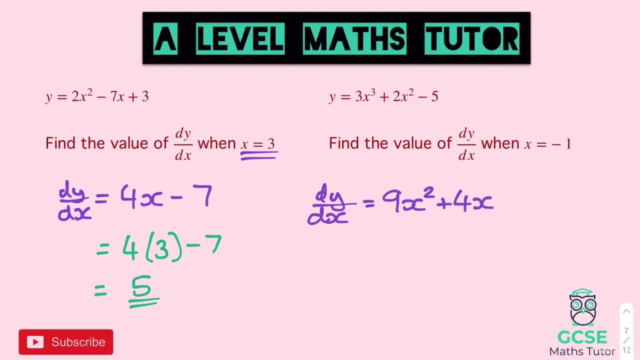 2 is 4, reduce the power by 1, gives us the power of 1, so 4x, And then the 5 times 3 is going to disappear, And again we've just got a value here. So x is minus 1, and we're. 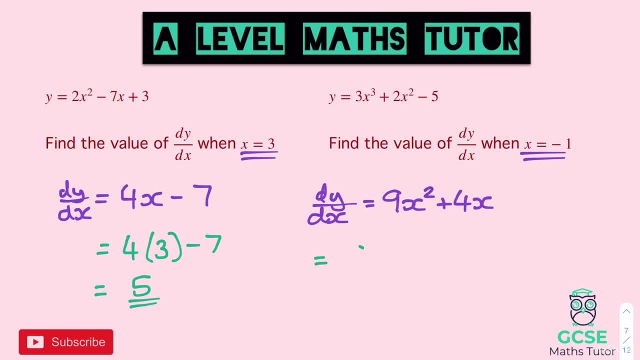 going to sub that one in. So let's sub that in and we get 9 lots of minus 1 squared plus 4 lots of minus 1.. Obviously, you can just type it straight into the calculator like that, but let's just go ahead and work. 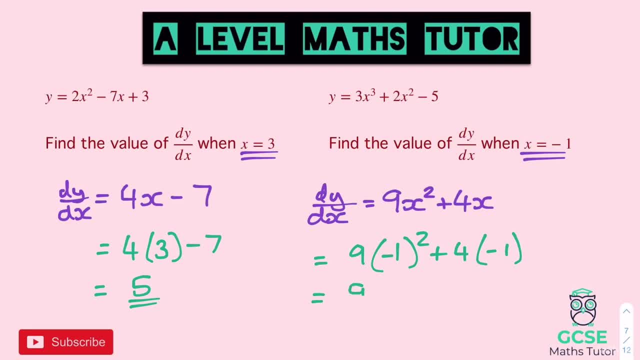 this out. So negative 1 squared is 1, times it by 9 is 9.. And then we're going to add to that 4, lots of minus 1.. 4, lots of minus 1, is minus 4, so it's 9. take away 4.. And again. 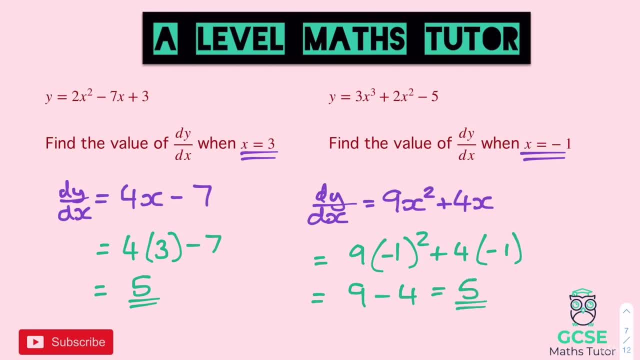 look, we get the answer 5.. So you've got the answer 5.. Subtitles by the Amaraorg community: both of these and there we go. that is our final two answers there. so what we're going to have a look at next is obviously differentiating some slightly harder pieces here, and let's have a look. 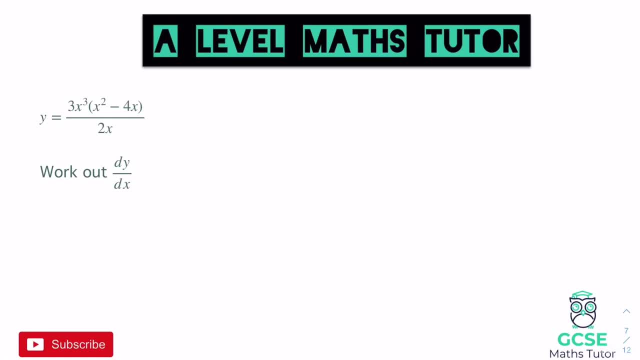 at that now. okay, so we've got one of these on the screen, so first things first. it doesn't look as nice, but let's just go about sorting out the top and then we'll discuss how to get this into a single line. now, when we're differentiating, we don't want to differentiate it while it's in a 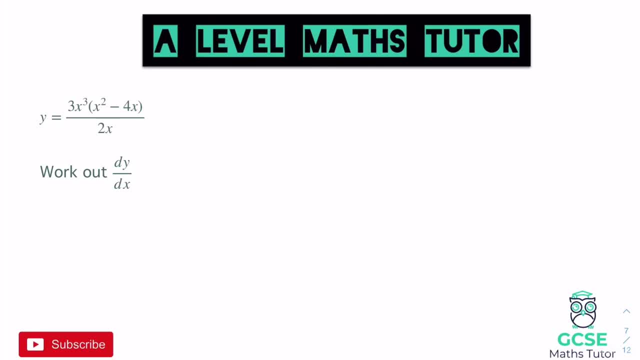 fraction. we want to get it down to a single line, so we're going to have a look at going about that. so if we expand the top, to start with, 3x cubed times x squared is going to become 3x to the power of 5- remembering to add the powers- and then on to the next bit, 3 times the 4, which is a minus. 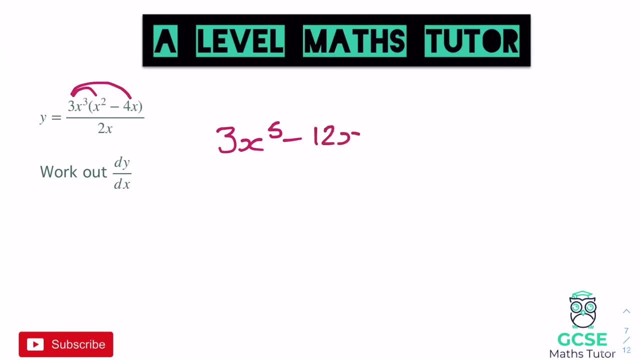 in the middle there, so that becomes 12. and then adding the powers gets us x to the power of 4. now that is all over 2x. now thinking back to obviously indice rules here, when we're dividing we can subtract the powers. now numbers are going to divide the numbers powers we're going to 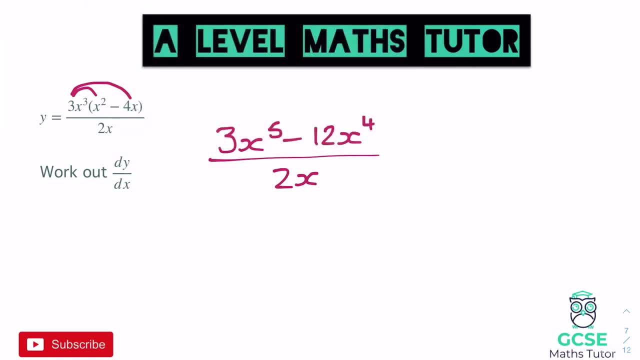 subtract them. so if we go about simplifying this, let's see what we get now. that's 3x to the power of 5 divided by 2x. now the 3 divided by 2 would give us 3 over 2. so we have 3 divided by 3 over 2. and if we subtract this power of 1, here for the x off, 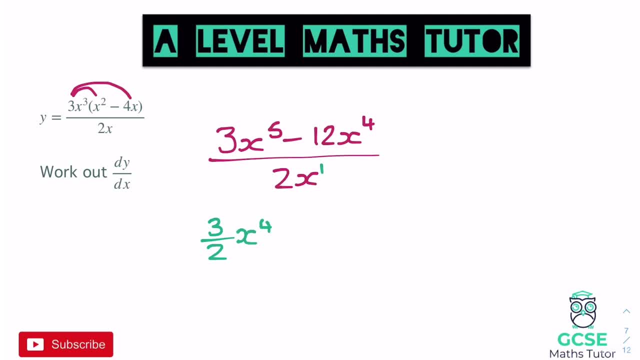 the x to the power of 5, we get x to the power of 4, so we get 3 over 2 or 1.5 x to the power of 4. we've got a minus in between. 12 divided by 2 is 6, and then we've got x to the power of 4. take away: 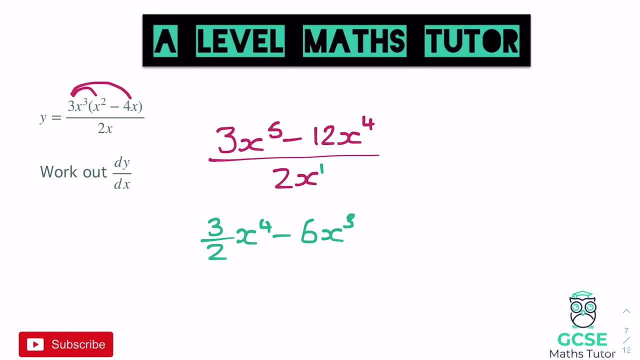 x to the power 1, which is x cubed. there we go. so that is obviously simplifying that down into a single line. so that's what we get now: that 3x to the power of 5 divided by 2 would give us 3 over 2. 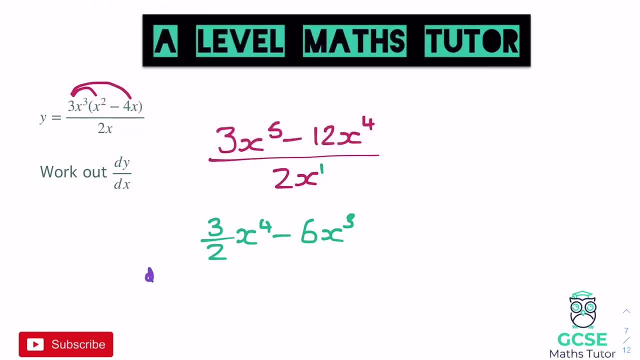 now we can actually go about differentiating this, so we can say dy over dx, and now we can just follow the same process. so 3 over 2 times that power of 4 becomes 12 over 2. okay, so we get 12 over 2 x to the power of 3 when we reduce it. take away 6 times the 3- there is 18x- and reduce the. 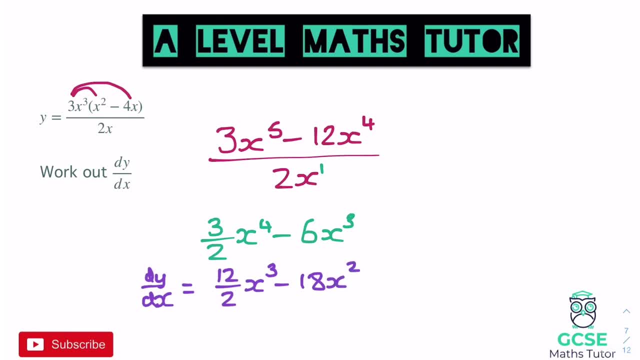 power down to a 2. now, obviously there's one thing here that we need to sort out, and that is that 12 over 2- 12 over 2- is 6, so we can get rid of that 12 over 2 and we can change that into a 6. there we go. 12 divided by 2 is 6, so there we go. that is obviously that differentiated now. okay, and obviously just a little process on how you can go about simplifying that down and making sure it's a single line first, but remembering all your rules of indices there, obviously taking away the powers and not being put off by the fact you know there's a fraction here. we could have fractions involved or, of course, you could write it as a decimal if you wanted to, but i'm going to be leaving it in fractions for all the ways that i'm going to go about some of these. but let's have a look at another one. 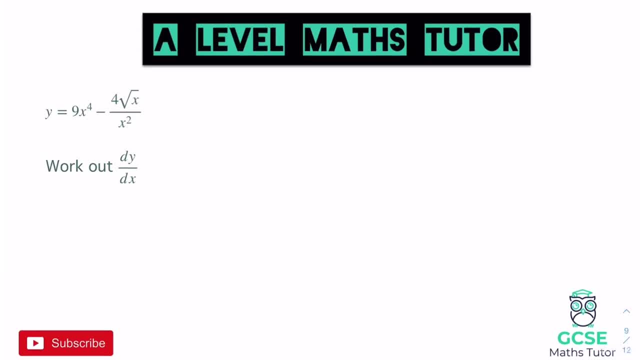 okay. so this one here does look- uh, you know- a lot nastier than the last one we just looked at, and that's primarily because we have this root x here. now, obviously, remember, when you have a root, there's another way of writing that as a power, and that is that the square root of x is also equal to. 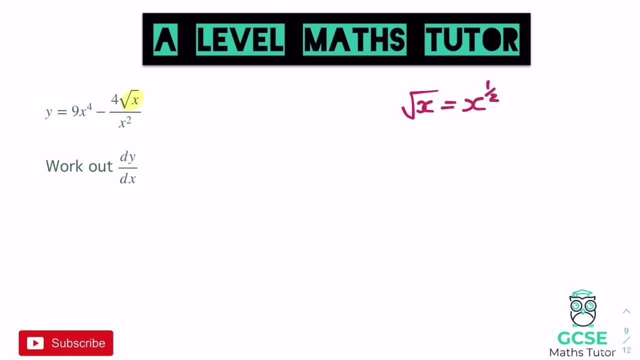 x to the power of a half. so don't be put off by a square root. it shouldn't throw you at all. it's just that we're going to write it in a slightly different way, and if we go about actually writing that, instead of writing it like that, let's write it as 9x to the power of 4. 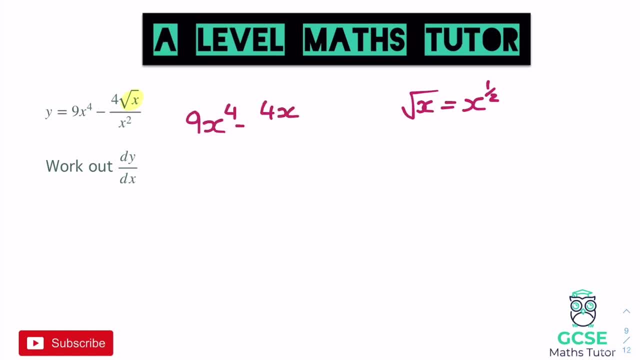 take away 4x to the power of a half divided by x squared. there we go, so that shouldn't really put us off. and now we can obviously get this into a single line because we can look at obviously subtracting this power of x from the one on the top. and if we do that, let's see what we get. we get 9x to the 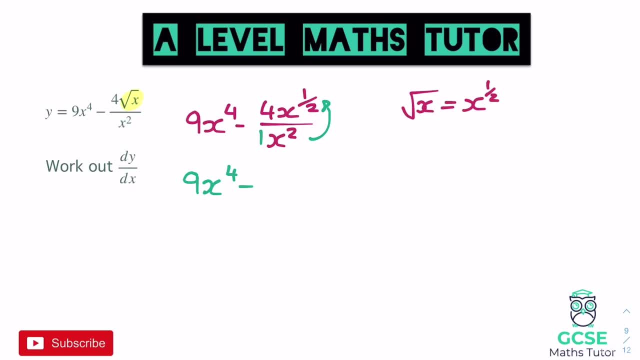 power of 4. take away now. technically there's a 1 in front of the x squared, so 4 divided by 1 is still 4 and we're still going to have an x and we've got to do a half. take away 2 now, obviously. 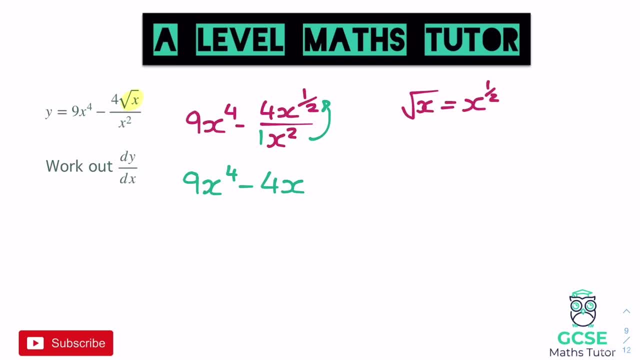 just a little thing here. obviously you can type that into your calculator. but 2 as a power in terms of halves, 2 is 4 halves. so we're taking away 4 halves from the one half and that leaves us with negative 3 halves, or 3 over 2. so there we go, that's obviously. 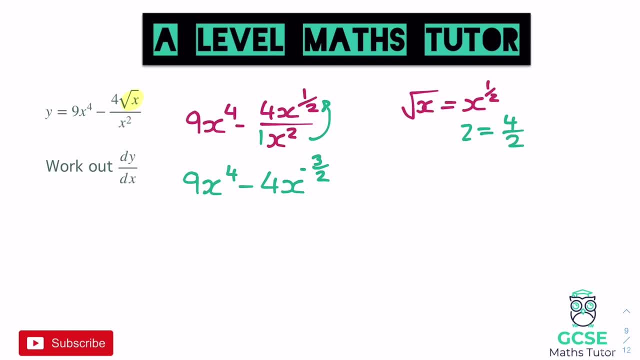 now written as a single line, obviously just subtracting the powers there when doing that division. and now we can go about actually differentiating this. so we get dy over dx and that's going to equal. and let's have a look: 9 times the 4 is 36x. reduce that down. 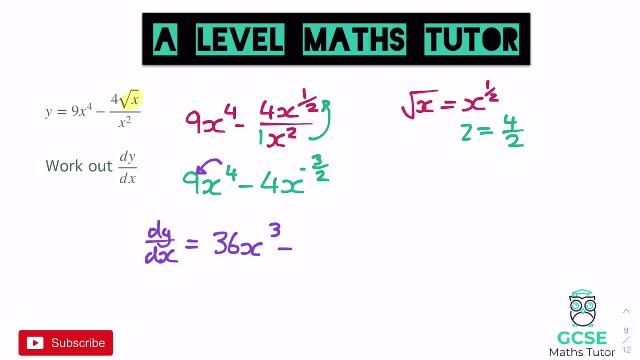 to a power of 3 and then we have negative 3 halves times negative 4 at the front. so that's going to become positive because we've got negative 4 there and we're going to times it by that negative power and that's going to become 12 over 2. 4 times 3 is 12 over 2 and that's going to be x. 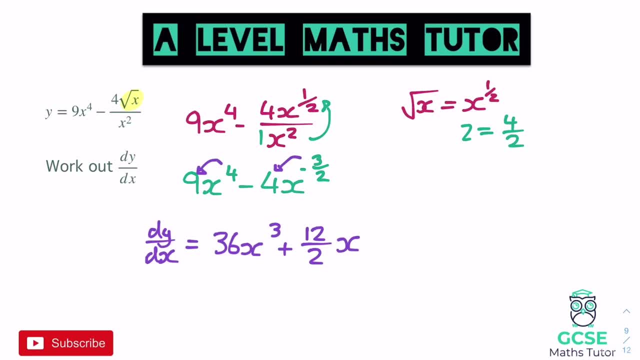 and if we subtract 1 from that power now, that's going to go down to minus 5 over 2. and there we go, just taking away 1 from negative, 3 over 2, or in essence taking away another 1 equals 2 halves, ok. 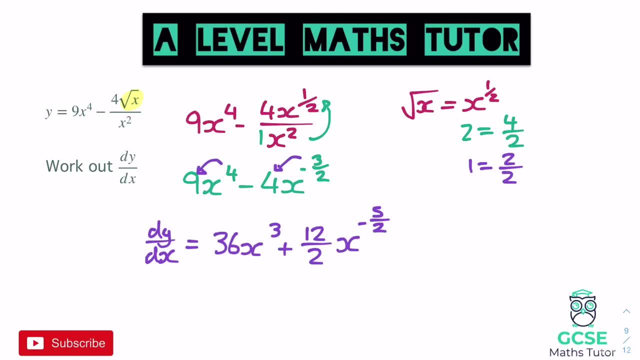 So taking away another two halves from that power. Obviously, you can type some of these into your calculator, But there we go. We should be able to hopefully do some of these without a calculator. Now there's obviously one thing to sort out. 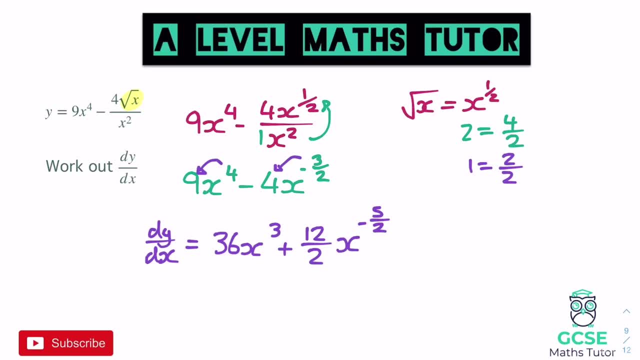 And that again is that 12 over 2 there, And 12 over 2 is a whole number, It's 6.. So we would write that as 6 there rather than 12 over 2.. So if we put that in instead, 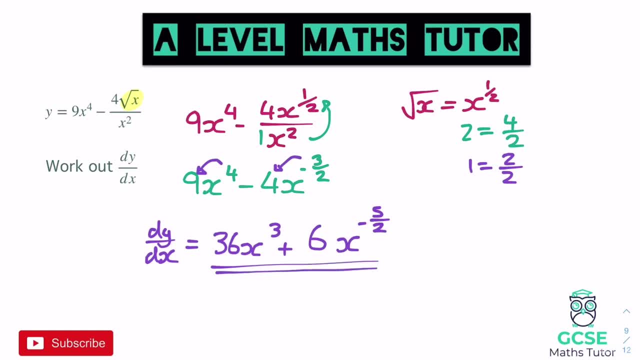 And there we go There. is that differentiated? OK? so hopefully just a few little questions there that just show you obviously not to be put off by some of these questions. Sometimes they don't look the nicest, But it's all about getting it into that straight line there. 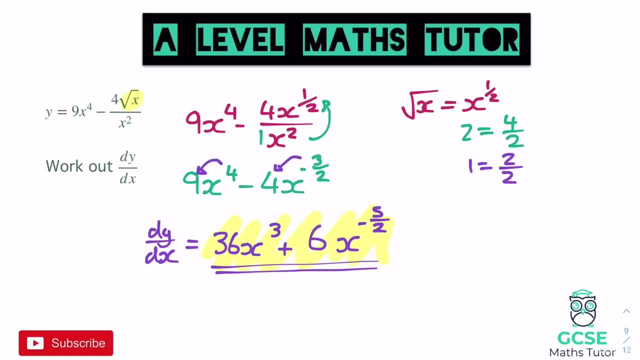 And obviously just being very careful with your powers when you multiply them by the coefficient And then reducing it by 1.. So there we go. Here's a couple of questions for you to have a go at. OK, so a couple of similar questions here. 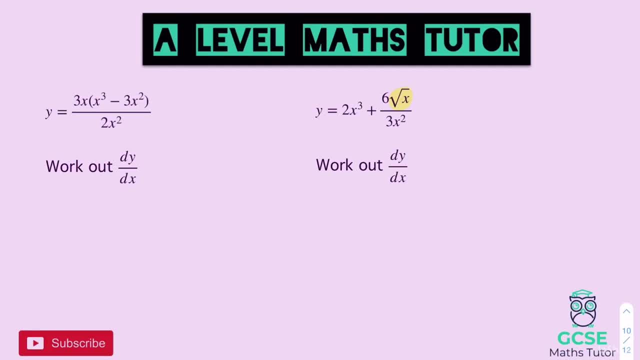 So obviously just watch out when you're doing these And just be careful that you rewrite this root x over here on that second question before you go about trying to get that into a single line. But there we go. Pause the video there. Have a go at these. 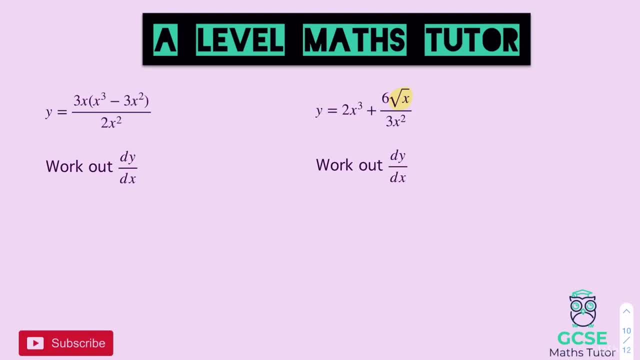 And we'll go over the answer in a sec. Right? OK, Let's have a look at these then. So for the first one, If we go about expanding that bracket to start with, we get 3x to the power of 4. take away 9x to the power of 3.. 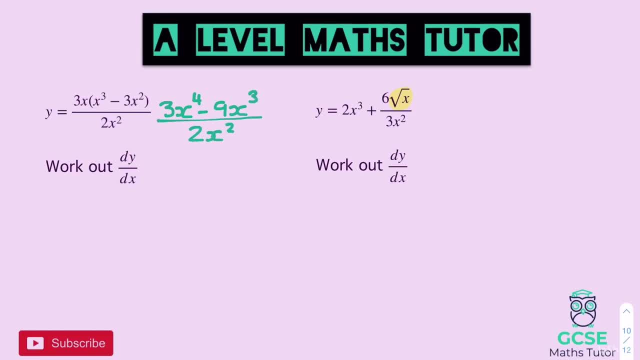 And that's all over 2x squared. Right now we can actually go about getting this into a single line. The first piece there, that's 3x to the power of 4.. If we divide that by 2, well, that becomes 3 over 2.. 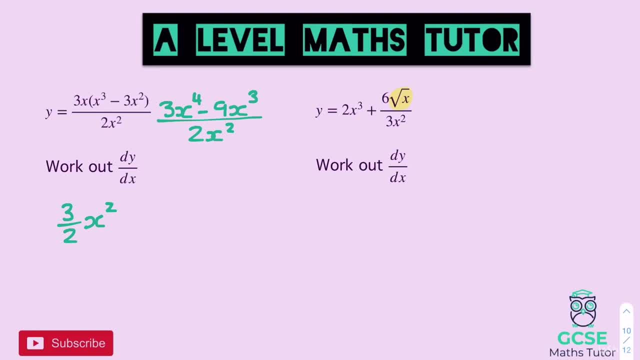 And the x goes down to the power of 2.. 4 take 2 is the power of 2. there Copy the symbol: the minus 9 divided by 2 is 9 over 2.. And the x goes just down to the power of x. 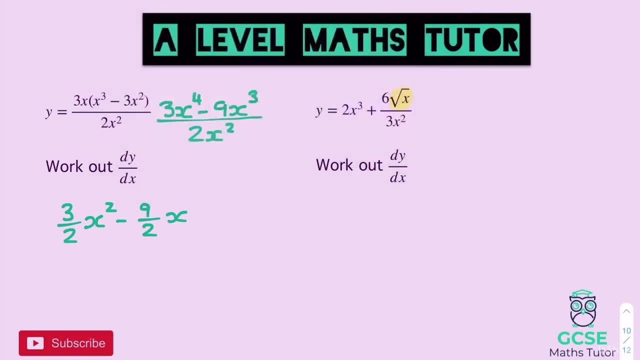 There we go. So it doesn't look the nicest, but let's go with it and just see what happens. Now we can go about differentiating. So we have dy over dx. Right, that first one. there we're going to do 3 over 2 times 2, which becomes 6 over 2.. 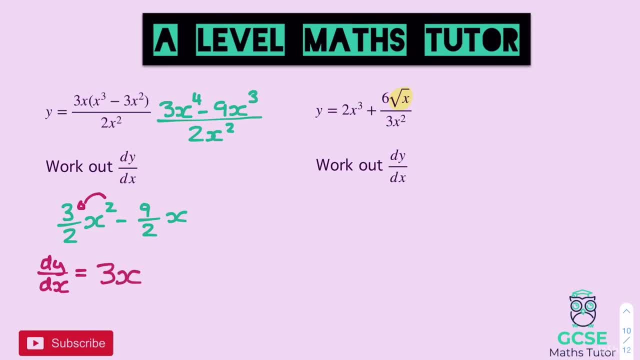 6 over 2 is 3.. So that's going to become 3x And obviously, reducing the power by 1, we've got 3x to the power of 1.. Then we're going to take away and obviously this power here is 1.. 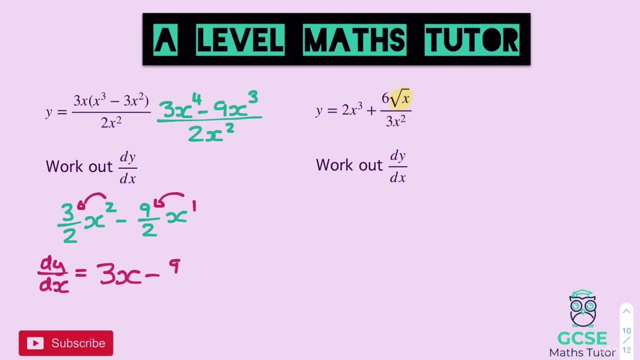 Multiplying that there by 1 gives us 9 over 2, or 4.5. And the x disappears. So we go 3x, take away 9 over 2.. And that is our final answer there, differentiating that one. 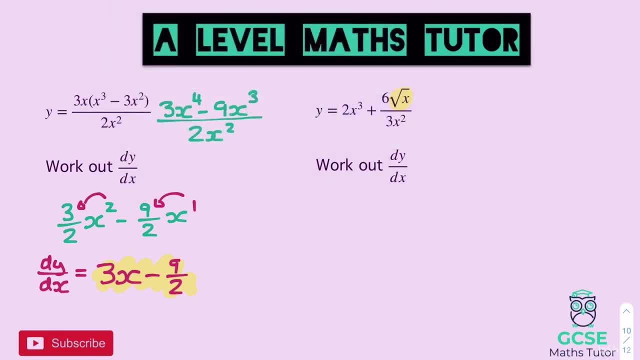 Let's have a look at our next one then. So obviously that first bit there, that root x, needs to be written as x to the power of 1 half. So let's rewrite this: So 2x to the power of 3 plus 6x to the power of 1 half over 3x squared. 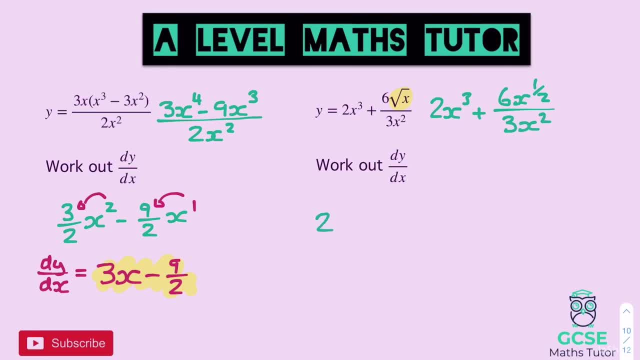 Now let's go about simplifying that there. Obviously, the 2x cubed doesn't need changing, That's already on a straight line there. And then we are going to add, And we've got 6 divided by 3, which is 2.. 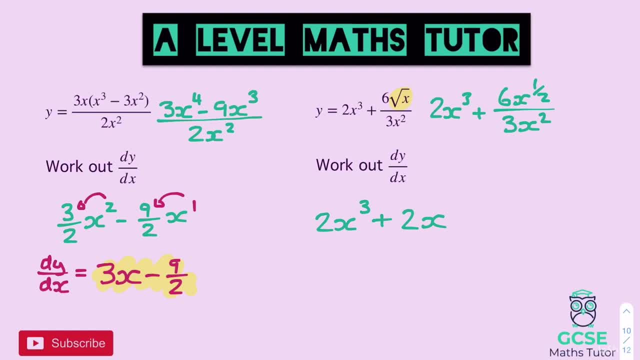 And then we've got x And we're going to do a half take away 2, which is minus 1 and a half, or minus 3 over 2.. Right, there we go. So now we can actually differentiate this. 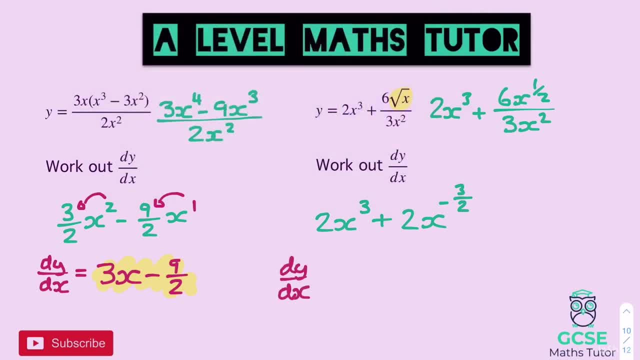 So dy over dx is going to equal. let's times the coefficient here by 3.. So we get 6x, Reduce it to a 2.. And then we're going to do the next one. Now, before I put that sign in, I'm just going to have a think about this. 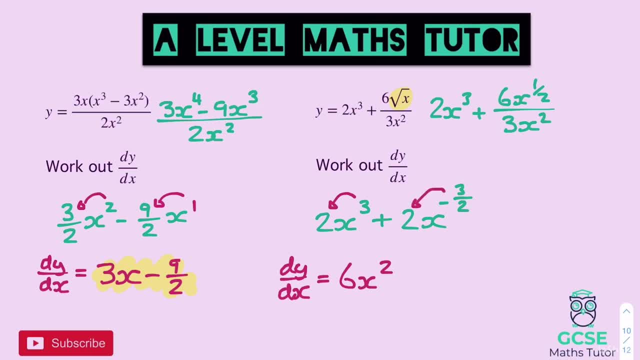 because I've got negative 3 over 2 times the 2.. So that's going to become negative 3 over 2 times 2 is 6 over 2.. 6 over 2 is 3. So that's going to become 3x to the power of- and take away 1 again, minus 5 over 2.. 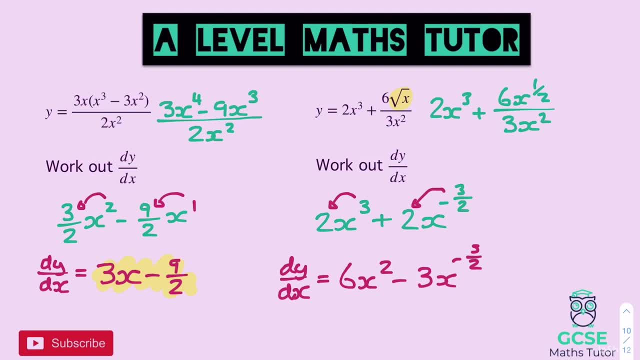 There we go. So we get 6x squared minus 3x, to the power of minus 5 over 2.. There we go, And that is that differentiated as well. Finish Finishing that one off. There we go. So there's the answers for those ones. 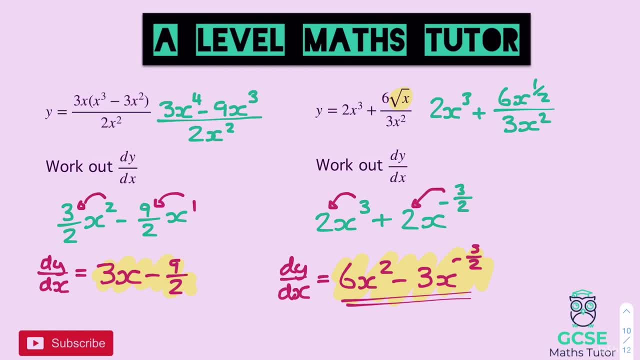 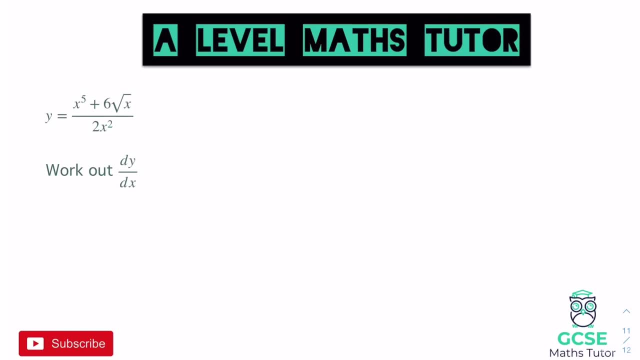 We've got one more question, obviously, that I mentioned at the start of the video, and that's the one we're going to have a look at now and see if maybe you're able to answer that one. Okay, so for our final question. obviously you saw this one at the start. 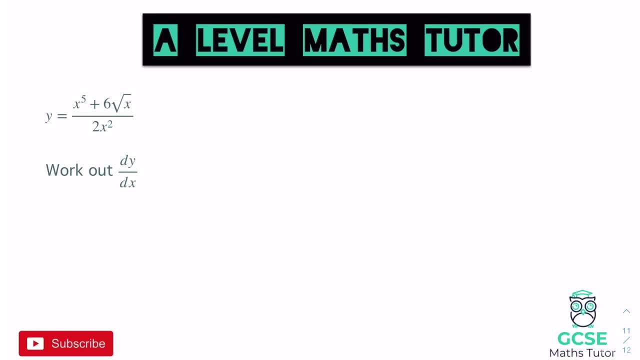 This is the one that you're going to have a go at, So obviously, pause the video there. have a go and we'll go over the answer in a sec. Okay, so this one here, obviously. what's different between this one and the last one we looked at? 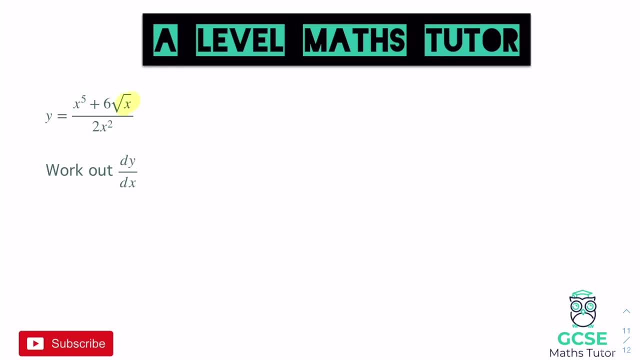 is. there's a whole fraction here, but we have this root x going on again and we need to sort that bit out first. So if I rewrite this, then we've got x to the power of 5 plus 6x to the power of a half. 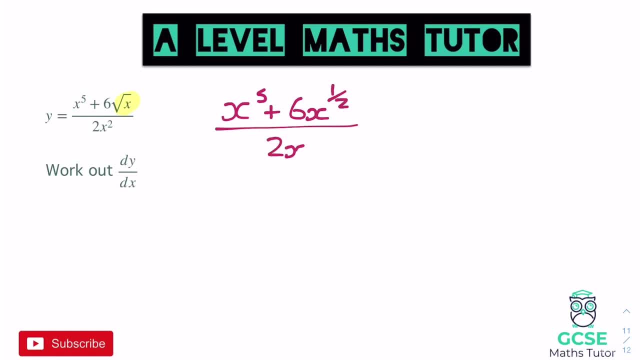 and that's all over 2x squared. Now, obviously, this can just be split up into two fractions, okay, So I could. if I wanted, I could write this as x to the power of 5 over 2x squared. 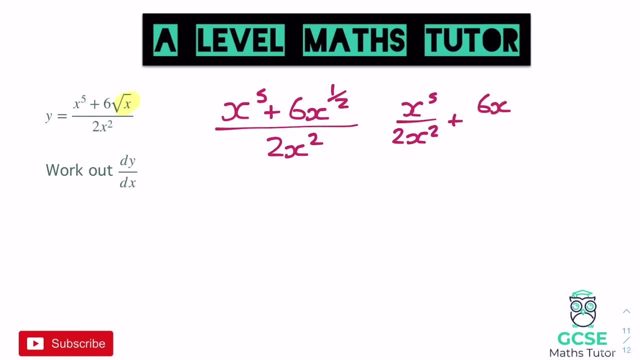 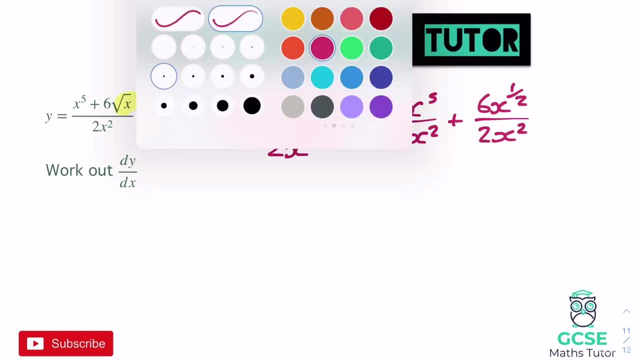 plus 6x to the power of a half, also over 2x squared. I didn't have to rewrite it as this and I like to look at it without doing that. okay, obviously, but we are dividing both, So we're just going to do both of these by the 2x squared. 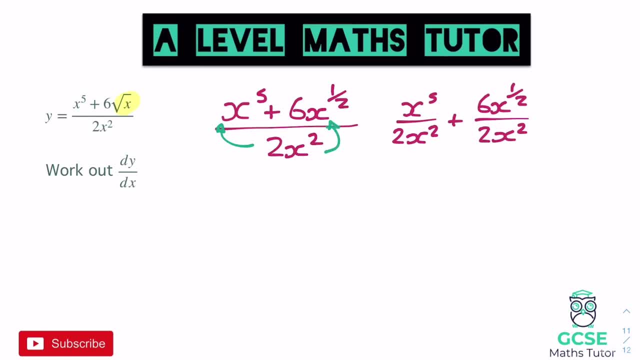 So we're just going to do both of those at the same time. okay, If you want to rewrite it, you can, but hopefully you're happy just to look at it as one big fraction. Now, x there obviously has the x to the power of 5, has a 1 in front of it. 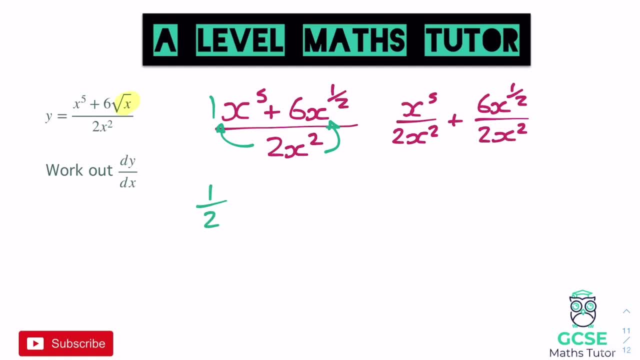 so 1 divided by the 2 there gives us a half, so we have a half x. take away the powers- power of 3, plus 6 divided by 2 is 3, so we get 3x and then a half. take away the 2, gives us the minus 3 over 2 that we've had before. 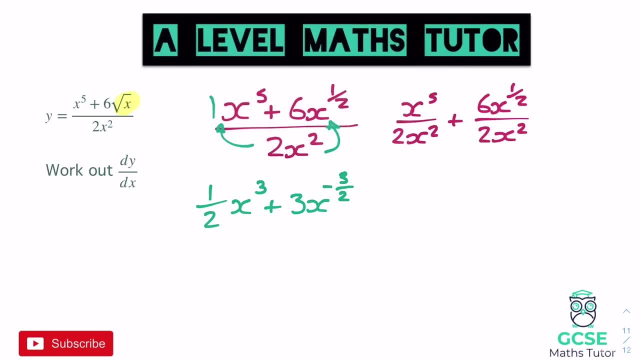 There we go, So that's in a single line. now, Now we can actually go about differentiating it. So let's have a look. What do we get? dy over dx equals. and then let's multiply that so we get 3 over 2,. 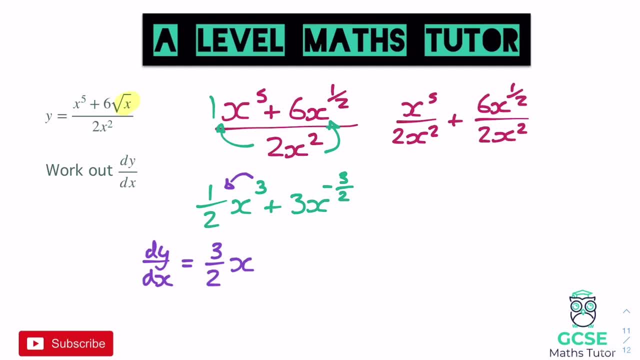 when you times a half by 3, so 3 over 2x, and reduce the power to a 2.. And then when we do the next bit, I'm not going to write that symbol in because it's a minus negative power, so that's going to become minus now. 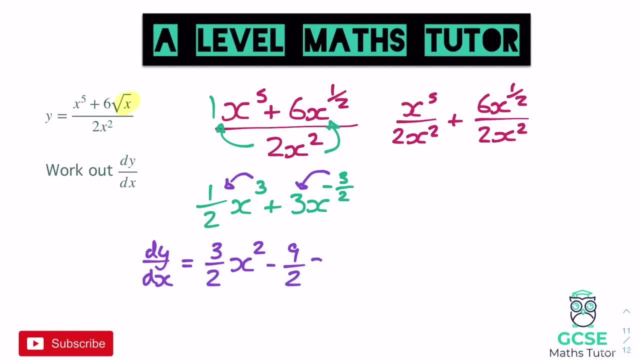 3 times 3 is 9, so it's 9 over 2x to the power of, and that is going to be minus 5 over 2 when we subtract 1 from that. Okay, obviously just subtracting 1 from the negative 3 over 2.. 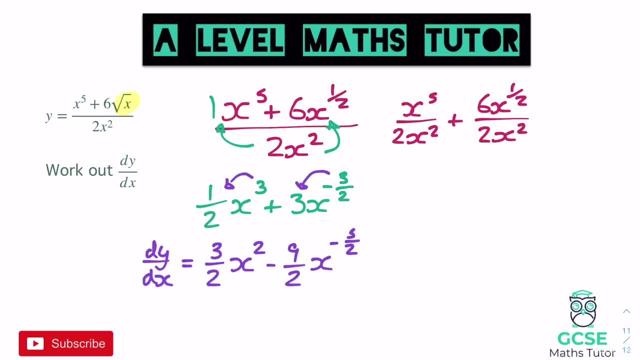 Right, okay, so there we go: 3 over 2x squared. take away 9 over 2x to the power of minus 5 over 2, and there's our final answer for this question, And hopefully everything that we've looked at there has built that up. 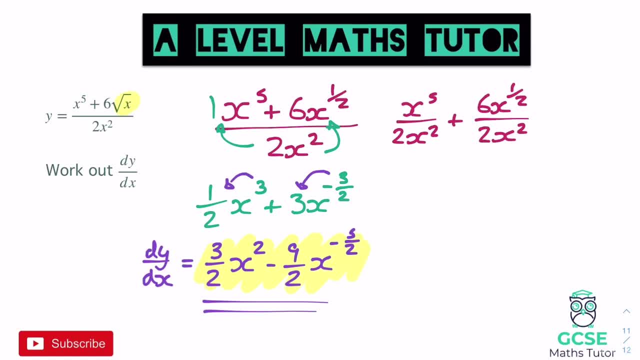 and all of this sort of question here makes sense now. Now, obviously that is the end of the video there. In the next one on differentiation, we're going to have a look at some slightly harder questions, but hopefully that's a nice introduction to differentiation for you there. 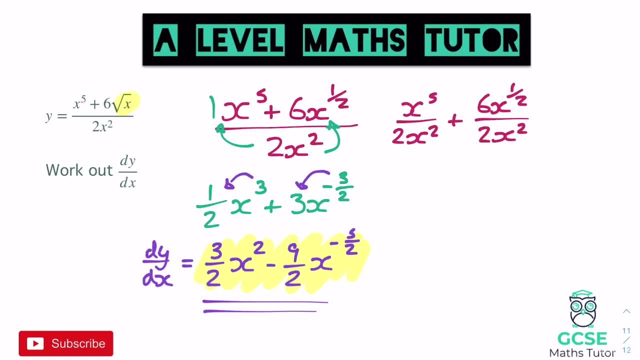 right up to this kind of question, which isn't an easy question. You know this is a nice challenge question here, But hopefully that's made sense and hopefully it was helpful If it was, please like, please comment, please subscribe. and I'll see you for the next one. 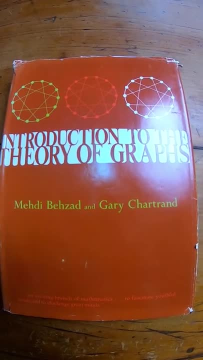 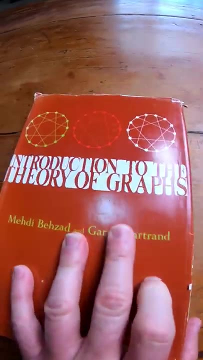 Introduction to the Theory of Graphs. This is the Chartrand book. This is supposed to be an introductory book on graph theory and it's pretty good. You can probably get an old copy for a few dollars. If you're trying to learn graph theory, I do recommend you know picking.